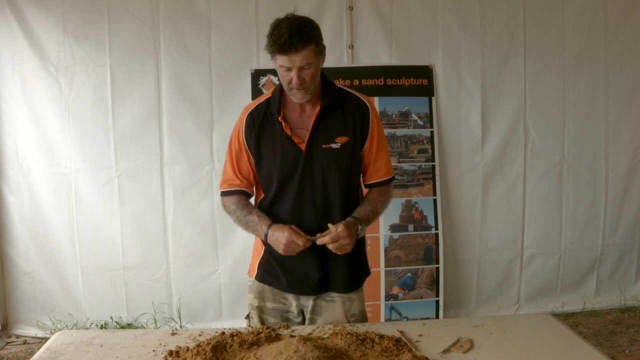 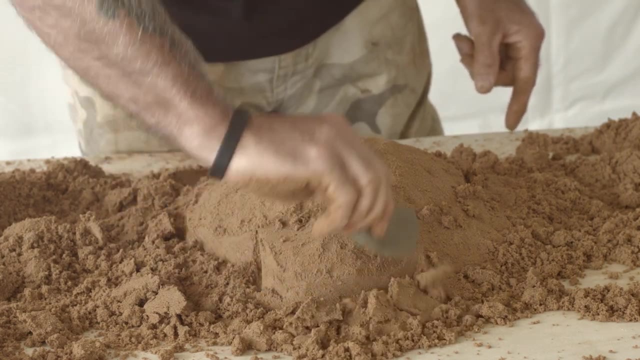 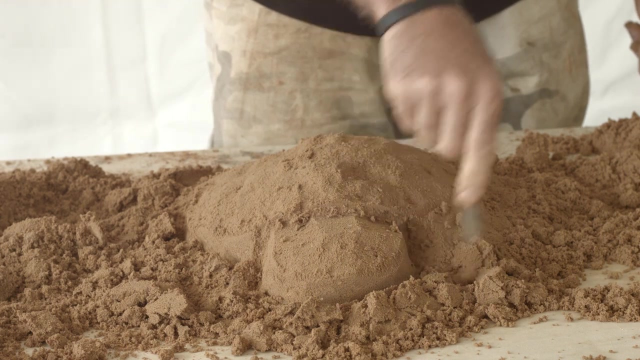 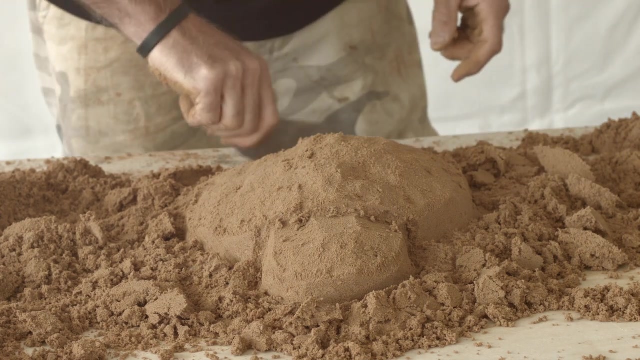 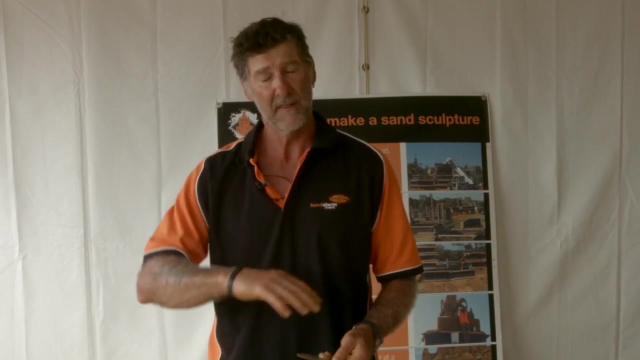 and smoothing the edges. So you hold the tool and you cut and you follow the line that you've already drawn. Step four is to smooth the sculpture out. So I'm doing a turtle, so we're going to smooth the shell out So you can smooth out the head, and then, once we've done that, then we'll get to step five. 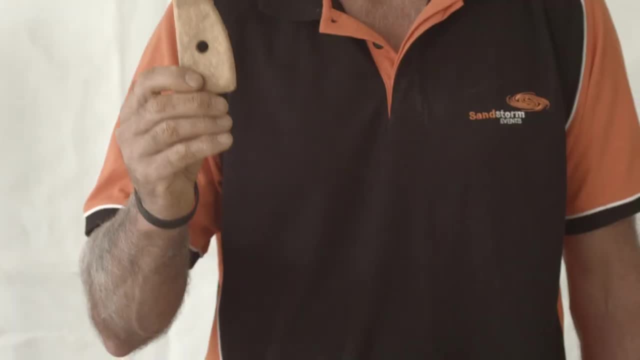 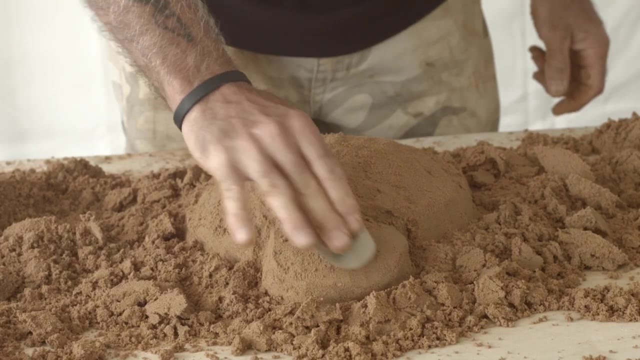 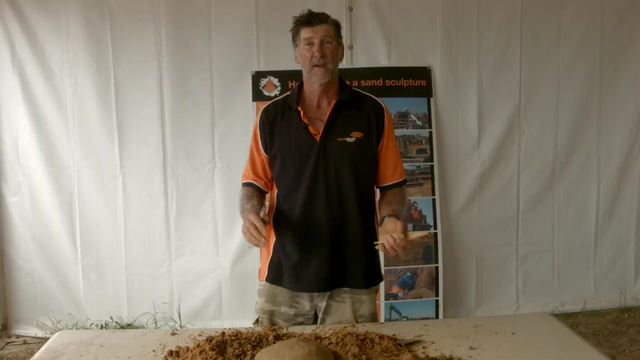 So you can use the tin tool, you can use the flat wooden tool that's provided, or you can use the knife to smooth it out like this. Step five is to add the detail to your sculpture, So you can use the various tools There's. 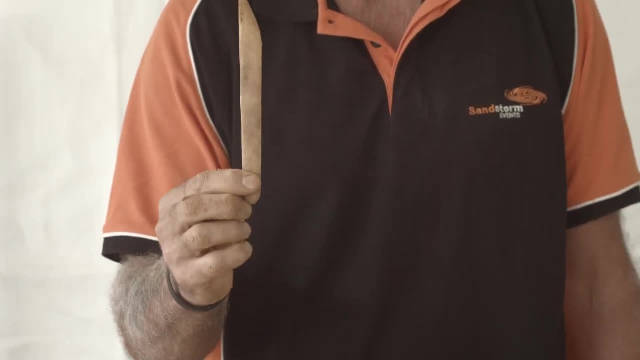 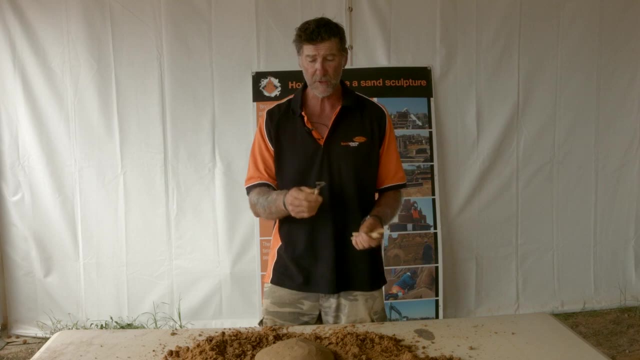 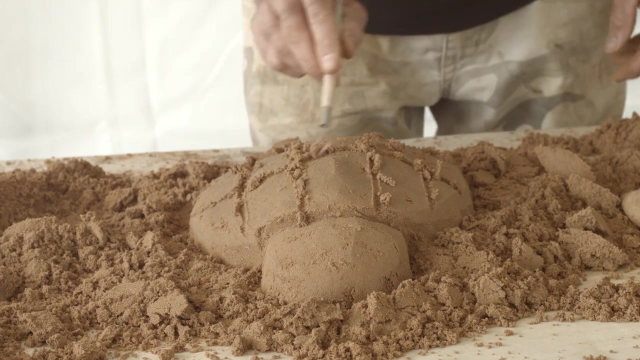 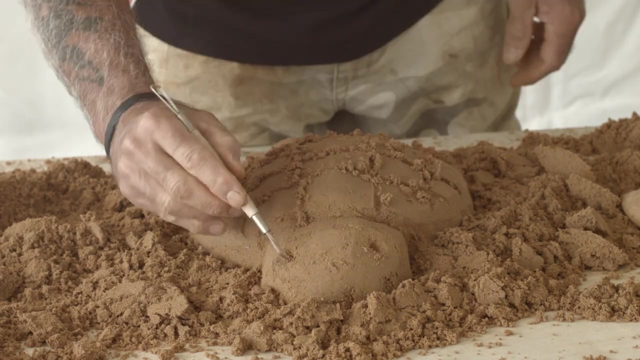 a wire tool. You can use your knife, You can use the wooden tools that are provided, and you can also use your tin tool. The best one for doing grooves is your wire tool. Always drag from the edge to the middle and just use the points. Don't use the whole wire. like this, You can clean up any of the excess by 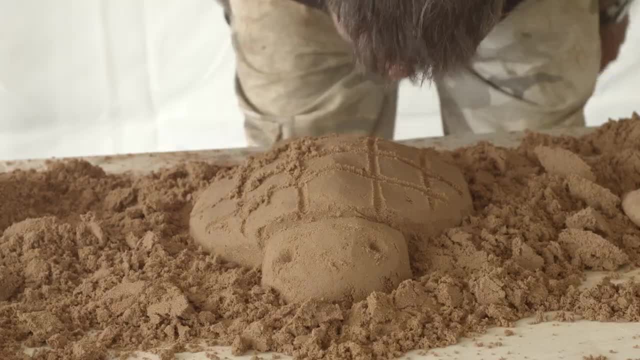 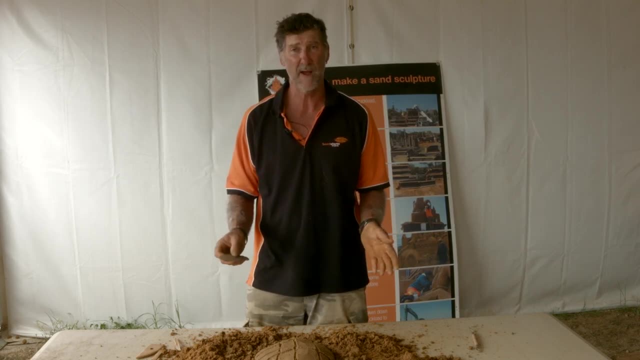 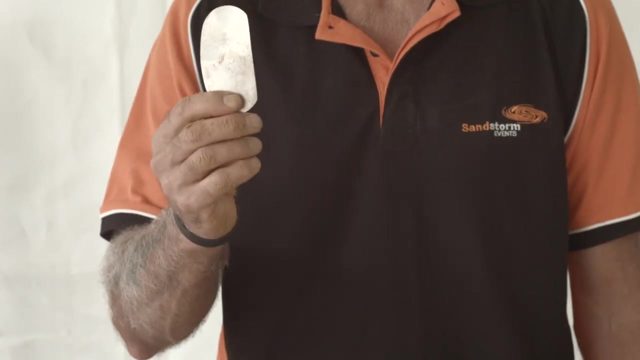 just quickly blowing over it. Step six is to clean around your sculpture so you can actually see what you've made, Because this is a turtle and he needs fins. we're going to make those as we do the step six process. So you use your tin tool to use the flat edge on the table. Clean around the outside Use. 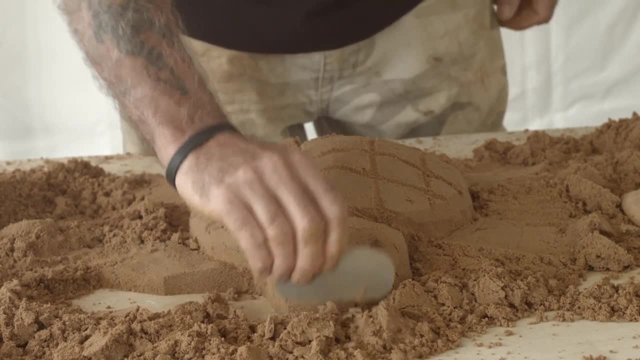 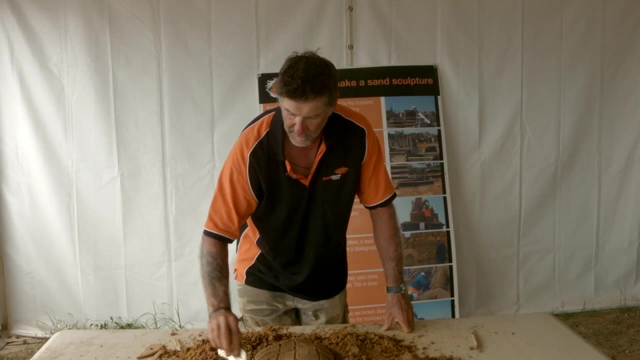 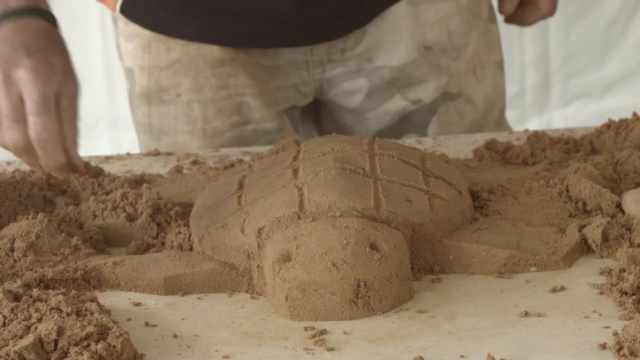 the bottom of the tool to actually push the sand away in a nice clean area around the sculpture you're going down. you can just smooth out a section of sand like you did originally, and you can just use the tin tool just to cut those out as you go. 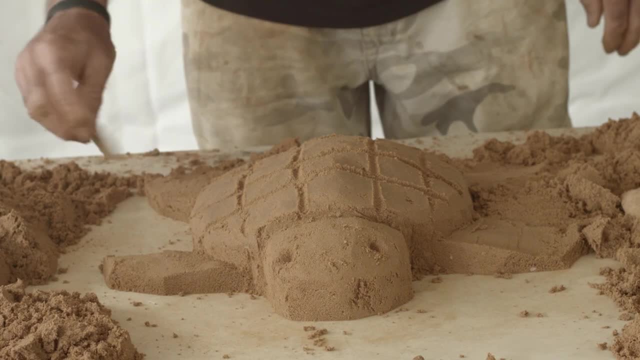 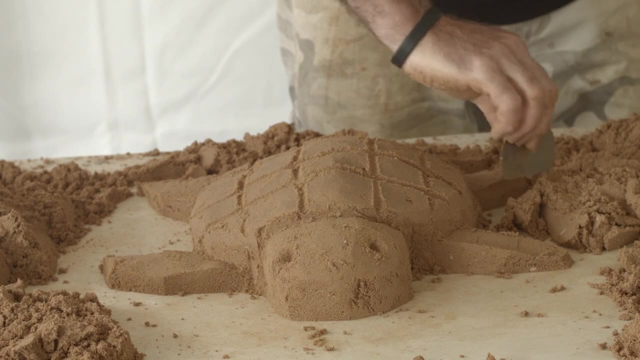 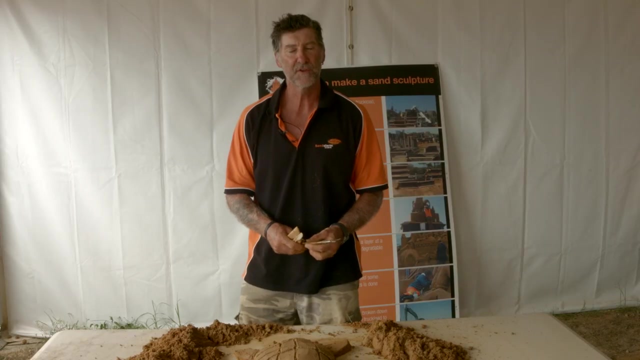 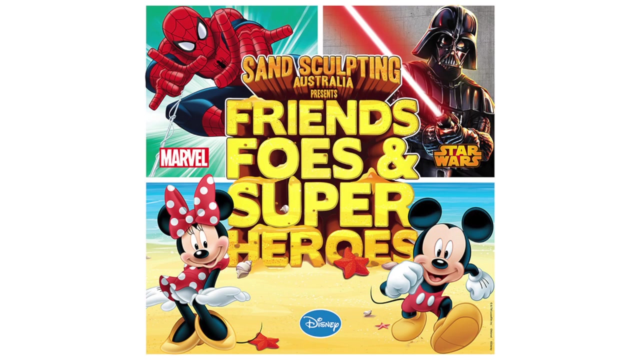 around and there you have it- a very quick turtle. the most important thing at the end is to actually clean around it. so you actually see what you've done. okay, thanks for watching this quick video on how to make a sand sculpture. get inspired, grab your tools and have a go yourself.